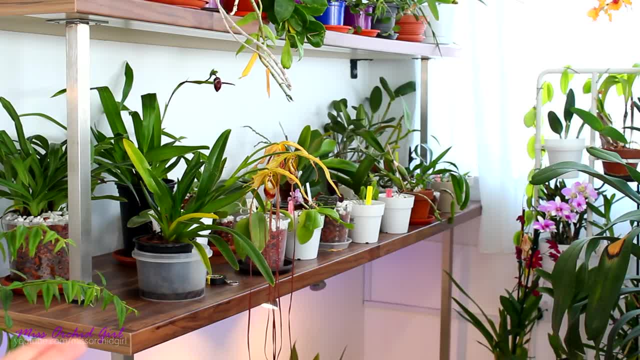 are just in between. But when we talk about low light orchids and high light orchids, we need to think in a balanced way. If a plant is low light, it doesn't mean it likes darkness, And in the same way, if a plant requires high light, it doesn't really mean it likes to stay. 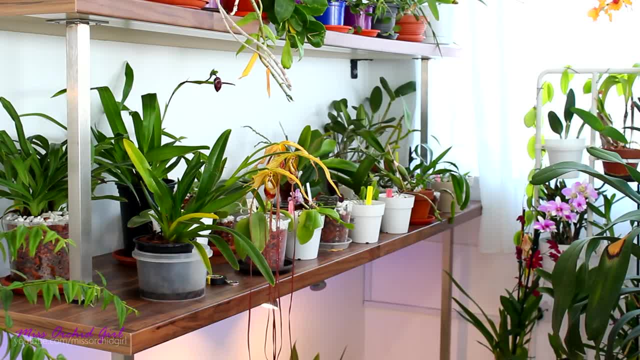 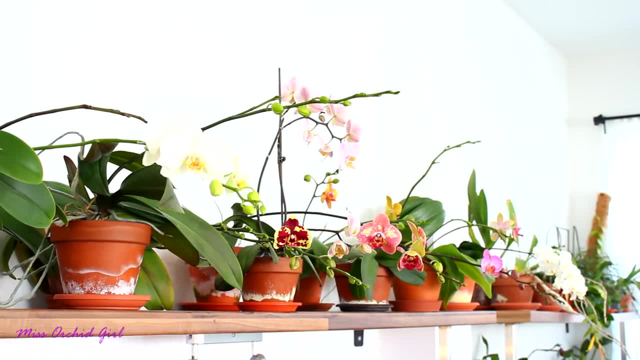 in full hot sun all the time. So let's start with the low light requirements. Let's start with the low light requirements. Give a few examples and see practically how much light they require. Alrighty, so the most popular low light orchid is the Phalaenopsis orchid, The one you find in 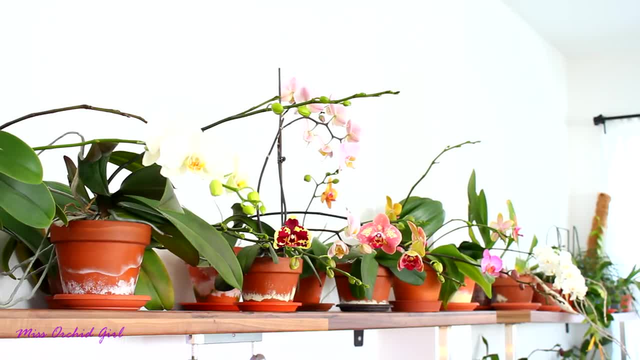 the stores or garden centers. Pretty much all stores have a Phalaenopsis orchid. Phalaenopsis orchids do not demand bright, bright light, But, as I was saying, they will not perform well in full darkness as well. So the fact that a Phalaenopsis is a low light plant doesn't. 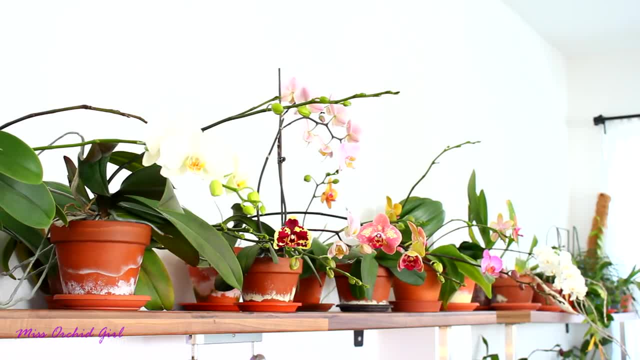 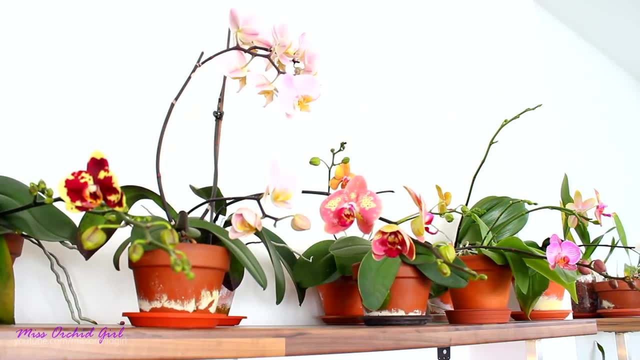 mean that we can put it on a shelf very far away from the window. So let's start with a window or under a desk and it will do just fine. No, actually it's not gonna do fine at all. What it actually means is that low light orchids can do very well if they never see direct sunshine. 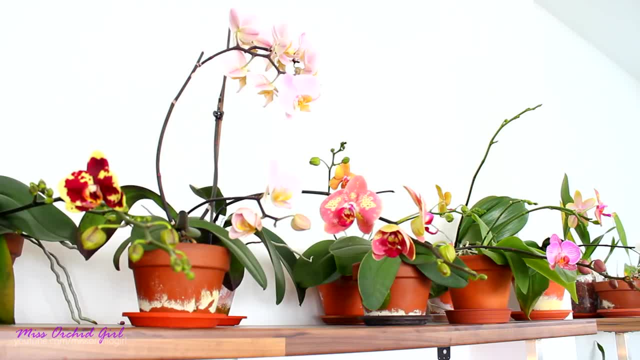 In practice, Phalaenopsis orchids do great in bright shade, And I think that is a better term to describe it, because shade means lack of direct sunlight, but it doesn't mean darkness. The way I grow my Phalaenopsis is on a shelf that never receives direct sunshine, not even filtered. 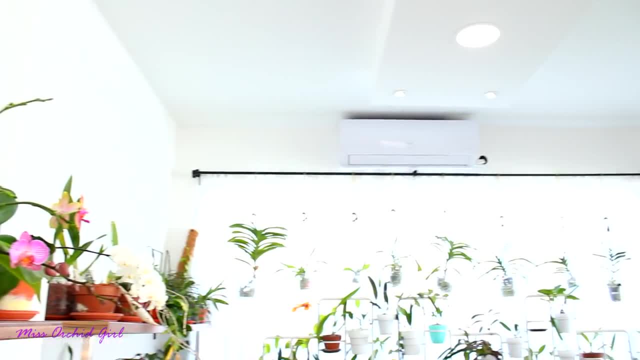 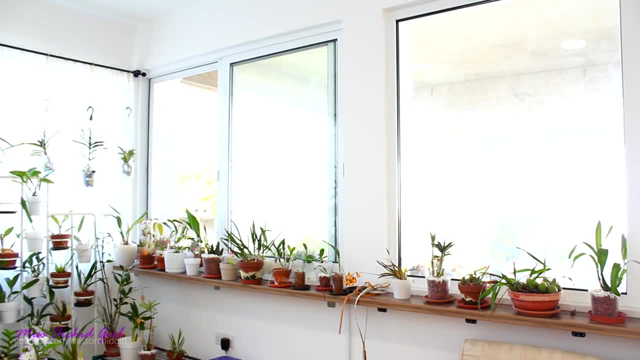 but doesn't have direct sunlight. So if I grow my Phalaenopsis orchid in a shelf that never receives direct sunlight, it does receive light coming from my southern window and not only also from my western window. In front of my greenhouse there is a white building which reflects light, So in my 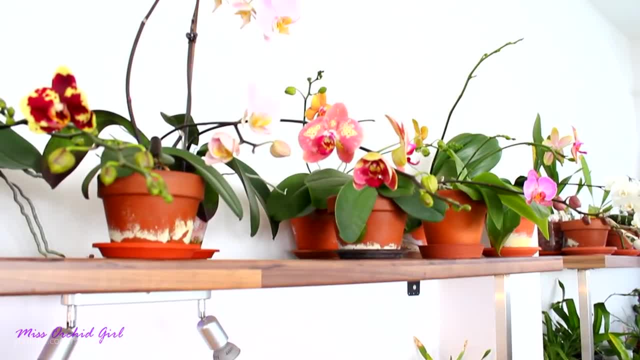 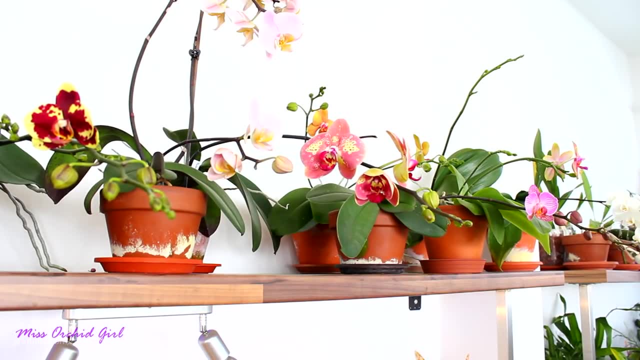 greenhouse there is quite a lot of bright light, which Phalaenopsis orchids really do enjoy, but they don't really require the sun hitting their leaves. So Phalaenopsis orchids will definitely do great near a bright window, but definitely in a place that doesn't receive direct sunshine. Some 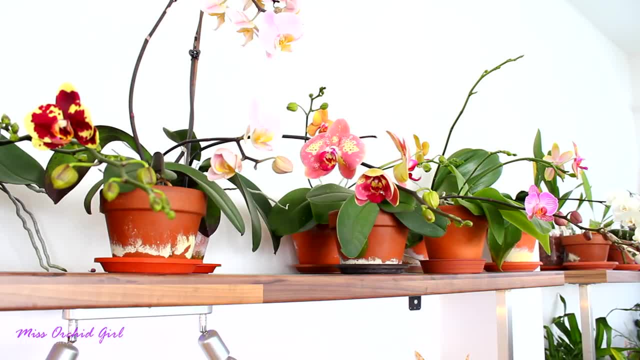 of my Phalaenopsis orchids did receive direct sunshine, but quite late in the afternoon when the sun was setting, and that is perfectly fine for them. What they cannot tolerate is direct, hot sunshine. on their leaves, Phalaenopsis orchids are pretty prone to having sunburns. 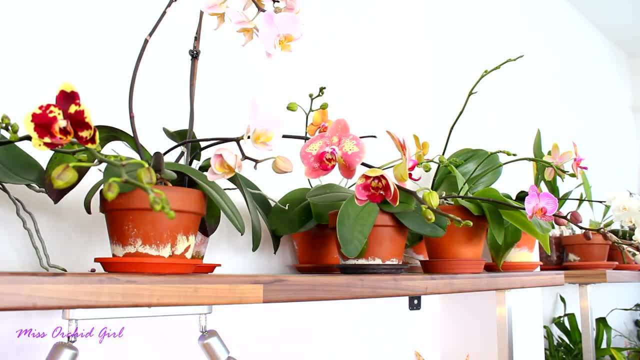 By offering light bouncing from the walls or coming from a bright window. we are still giving light so they can photosynthesize, but we are avoiding the possibility of leaf burns. So a Phalaenopsis orchid is a great orchid for those houses which do not. 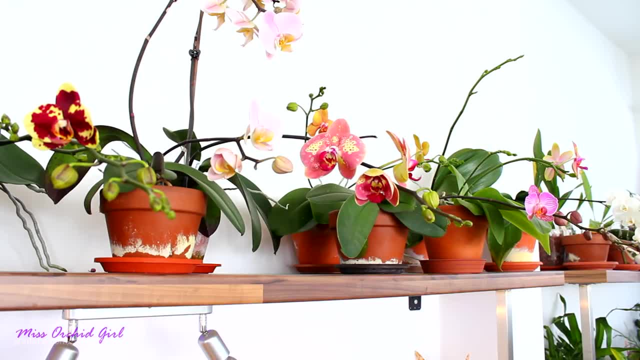 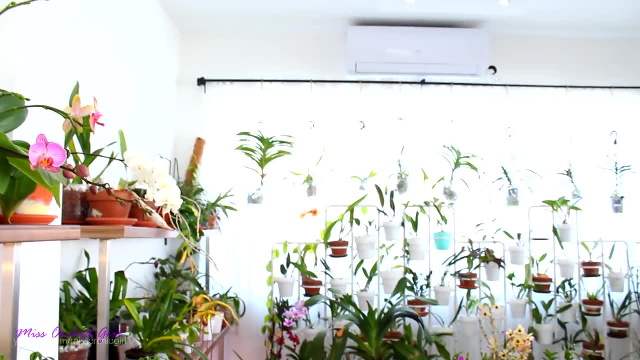 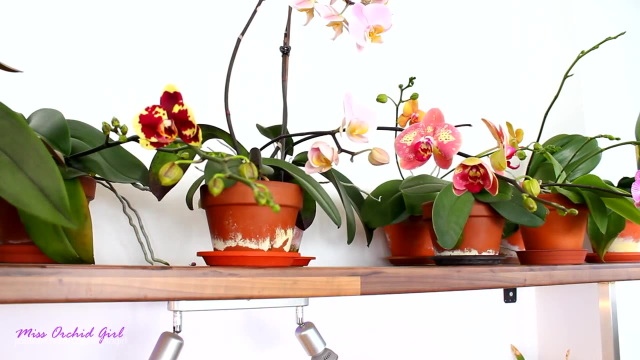 from direct sunshine, necessarily, but do have some locations in which sun either bounces from a fence or from another building, or in a room that has drapes, like I have, which benefit from direct sunshine and light up the room, Being that they do not require direct sunshine. Phalaenopsis orchids. 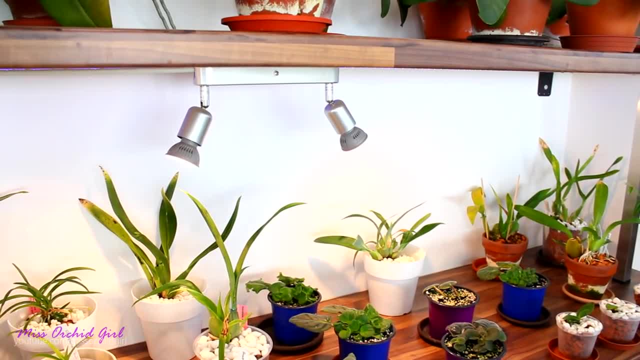 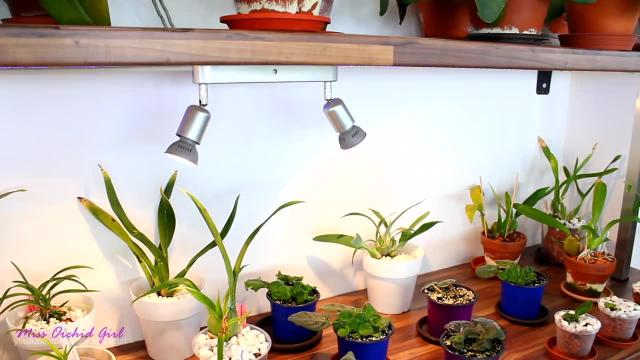 are also very good candidates for artificial light And here I have a setup with some LED spotlights and some other plants, but definitely Phalaenopsis orchids will do great in artificial light. In this, burning of the leaves can only occur if the leaf actually touches a hot bulb. LED fixtures don't. 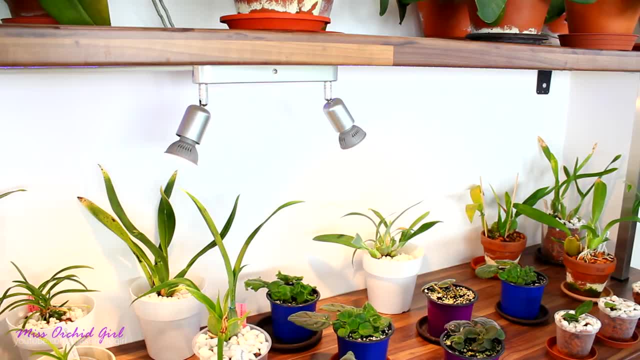 get all that hot, but it's still a good idea not to let the leaves touch the fixture. Other than that, it is pretty impossible to leaf burn a Phalaenopsis orchid, or any type of orchid, if we keep it under artificial light at a sufficient distance from the actual bulb. Generally low-light orchids, which 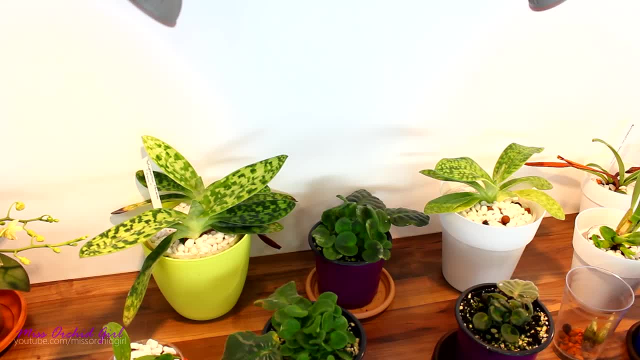 do not require direct sunshine. on their leaves do great under artificial light and, of course, in bright shade conditions such as paphiopedilum, Paphiopedilum, orchids, especially the complex hybrids that we can find in the stores- or flower. 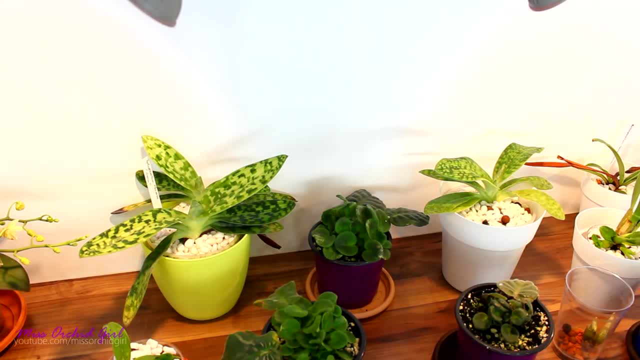 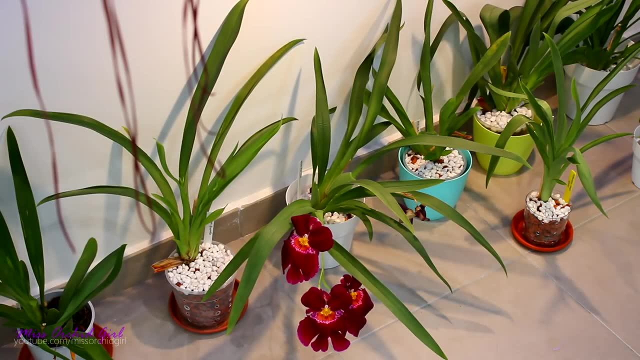 shops do not demand direct sunshine and can do perfectly well next to a Phalaenopsis or in the same light conditions. Meltoniopsis, orchids and the famous Nellie Eiler, which again we can find easily in stores or garden centers, are low-light plants as well, So they can grow and perform. beautifully, even if direct sunshine does not touch their leaves. They can do great in bright shade and also under artificial light. If they do receive direct sunlight early in the morning or late in the afternoon, there's really no problem, because the main thing we are trying to avoid is leaf burn, and low-light orchids generally are more sensitive to obtaining. 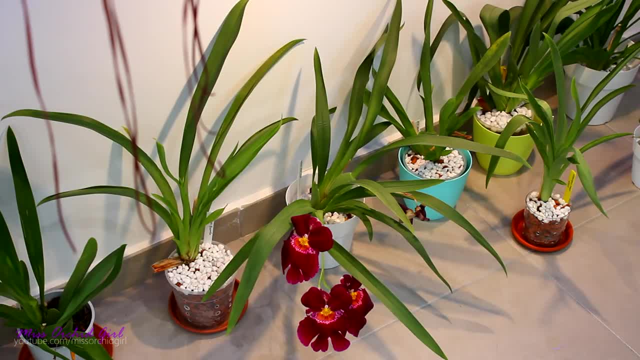 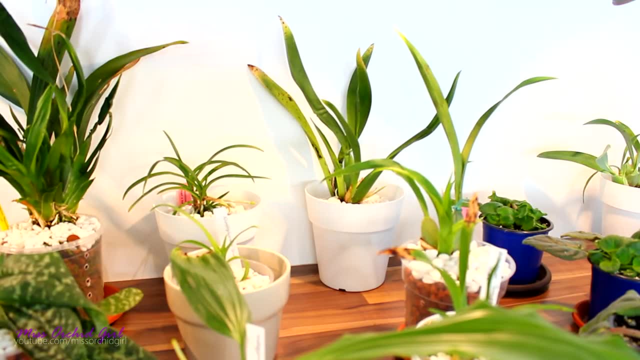 burns on their leaves because of sun, rather than medium-light orchids or high-light orchids. Now, medium-light orchids are somewhere in between high-light orchids and low-light orchids. They will not necessarily perform to their full potential in the same light conditions as 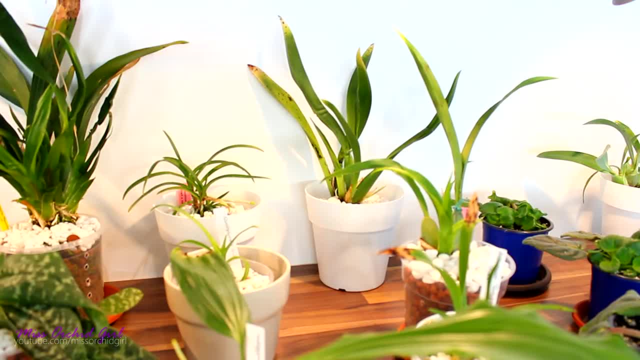 Phalaenopsis and paphiopedilums. Direct sunshine in the morning and late afternoon is actually very beneficial and in some cases, can make the difference between an orchid which doesn't want to bloom and one that blooms nicely. However, when it comes to 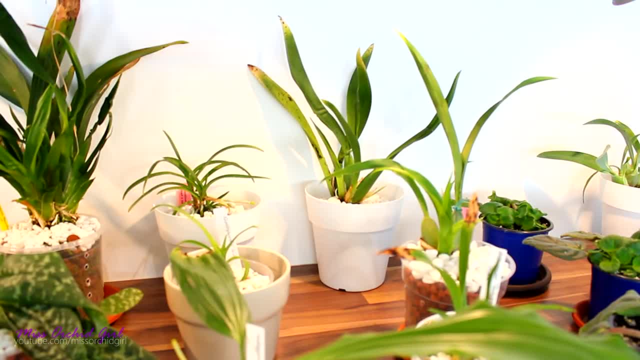 the time frame in which they need direct sunshine. they really don't need a certain amount of hours of direct sunshine. With medium-light plants we can do very well in bright shade conditions, but this bright shade needs to be a little brighter than in the case of Phalaenopsis. 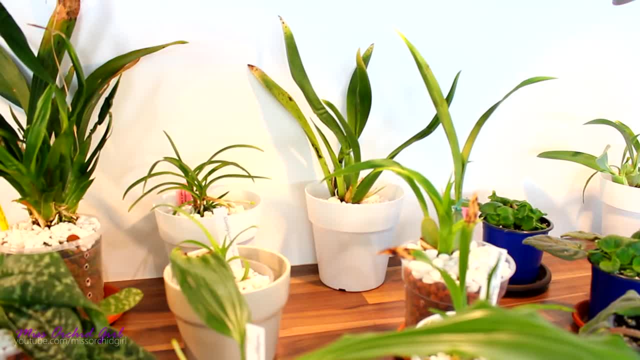 so positioning a medium-light orchid closer to the window will actually provide a brighter light intensity without actually providing direct sunshine. But with these orchids, if we can provide direct sunshine at a time of the day when the sun is not very hot, it's actually extremely beneficial. The most famous medium-light orchids are: 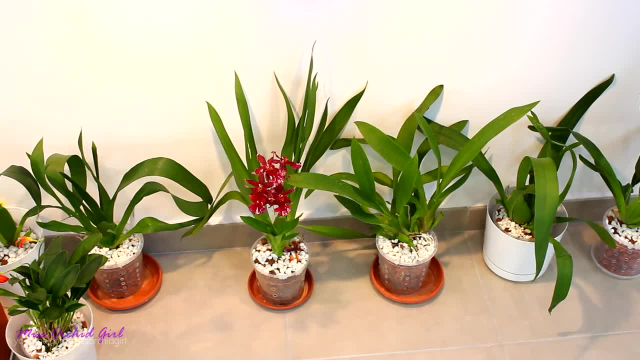 Oncidiums, or at least some Oncidiums- Meltonia, orchids, and, mind you, do not confuse them with Meltoniopsis And PS. I have a video on how to make the difference between the two in the. 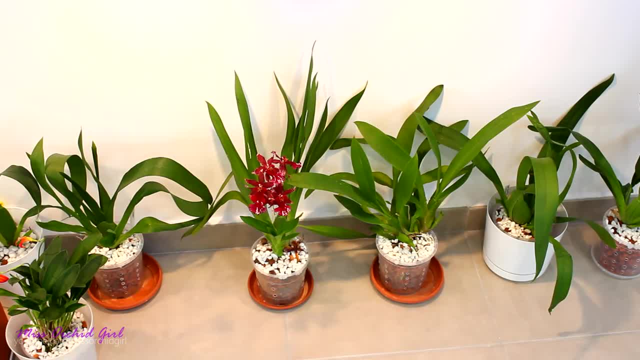 description below. so if you ever wonder, just check the description. And other Oncidium intergenerics are hybrids, even Brassia orchids. Medium-light orchids can do very well under artificial light as well, but we can adjust the intensity simply by placing the light closer to the orchid itself. 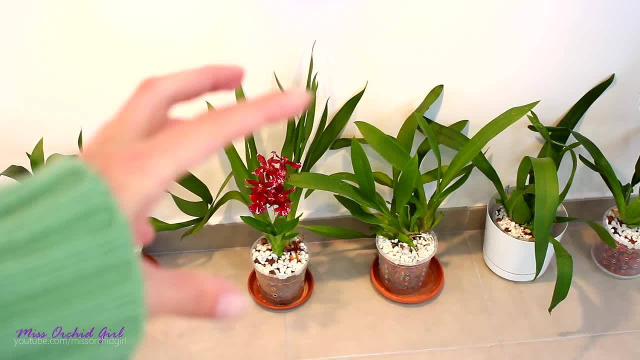 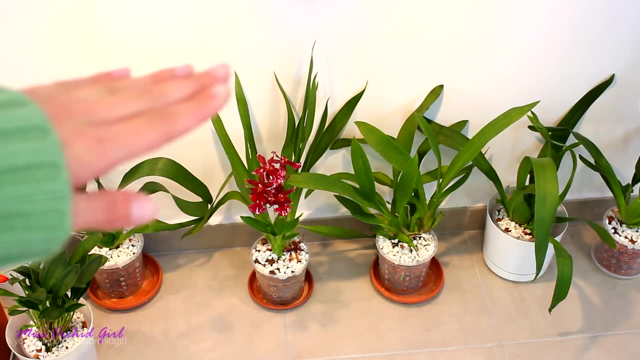 In the case of Phalaenopsis orchids, we can do very well from a light source which comes from the ceiling, but in the case of Oncidiums and medium-light plants, the artificial light source needs to be quite close to the orchid. And my light source is actually attached to the shelf. 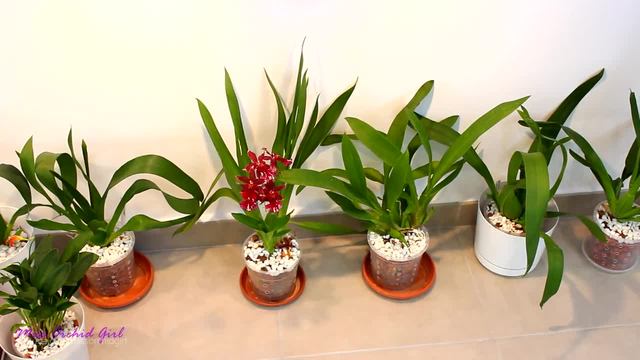 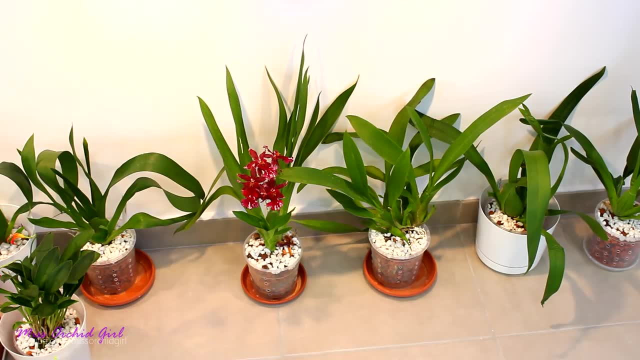 they have above them. so the distance in between them and the distance between them is very important, And the artificial light is about 20 or 25 centimeters. You can even go a little closer than that. As long as the leaves don't touch the actual bulb, everything should be okay. 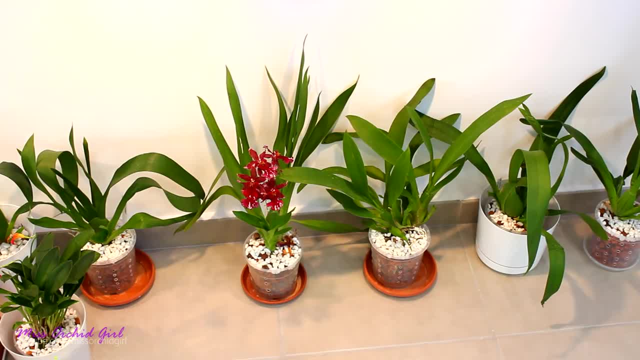 Furthermore, my medium-light orchids do receive direct sunshine, but again, it is later in the afternoon. Even if they do require more light than low-light orchids, they are still prone to getting sunburns because they are not adapted to a lot of sunlight. 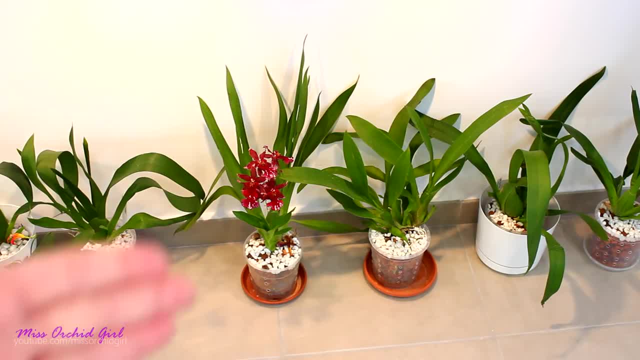 With medium-light orchids. there are also exceptions, even with Oncidiums. There are those types which do require brighter light and of course there are those hybrids or other species which can do very well in low-to-intermediate light conditions, But generally for medium-light orchids. 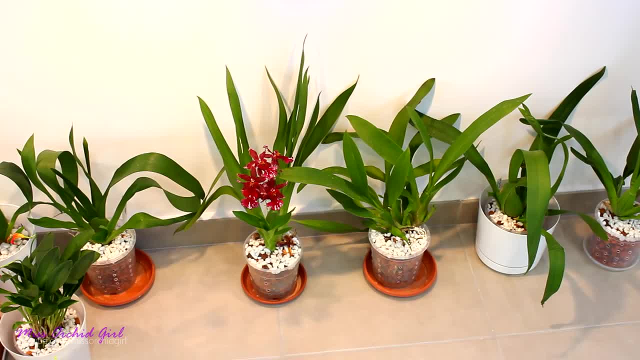 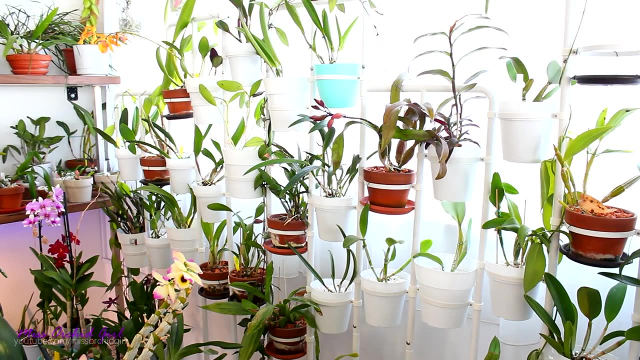 direct sunshine in the morning time or in the evening is very beneficial. They do still require sheltering from hot sun, but they are not as prone to sunburns as Phalaenopsis are or other low-light plants. And finally, the high-light orchids. These are the orchids which demand the 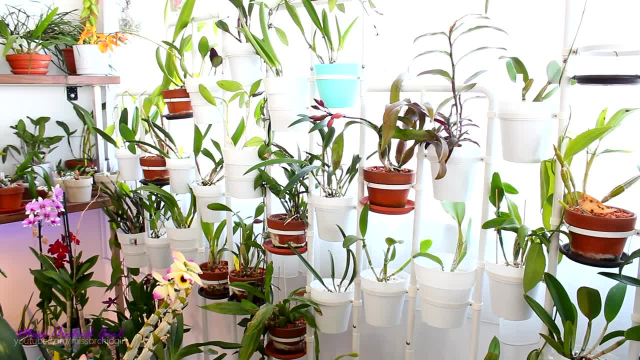 highest amount of light. These are the orchids which require the highest amount of light. These are the orchids which require the highest amount of light. These are the orchids which demand the highest amount of light. But, as I was saying in the beginning, it's never good to offer extremes, especially if an orchid is. 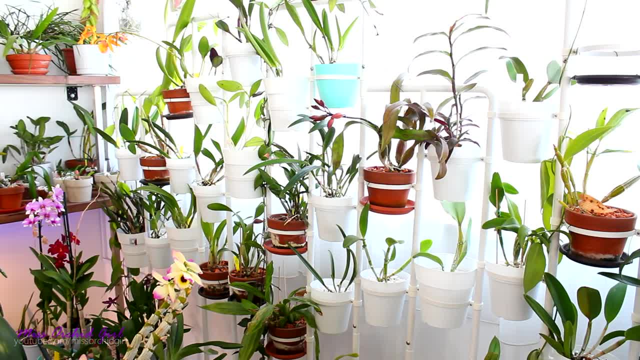 not gradually adjusted to the quantity of light. The high-light orchids can tolerate direct sunshine, depending on the species, but yet again, this category is quite diverse. Some orchids will tolerate more sunshine or hotter sunshine, while others will only tolerate filtered sun. The highest 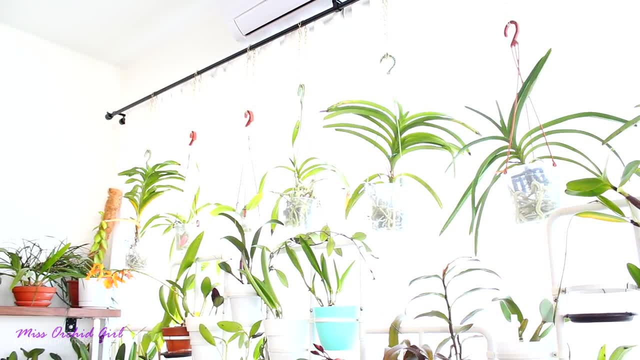 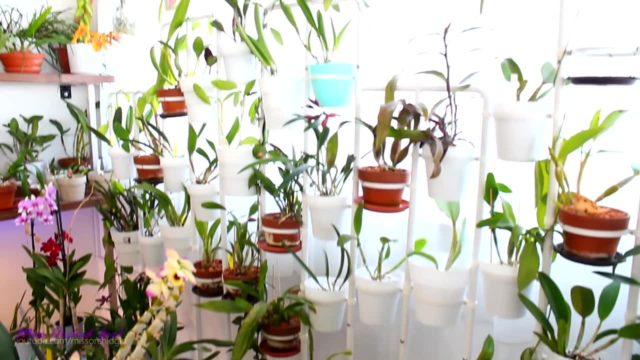 light orchids are definitely the Vanda orchids, which are famous for their light demand And under certain conditions, they can definitely tolerate direct sunshine. Other high-light orchids include Catlea orchids, but the difference is they don't require as much direct sunshine as 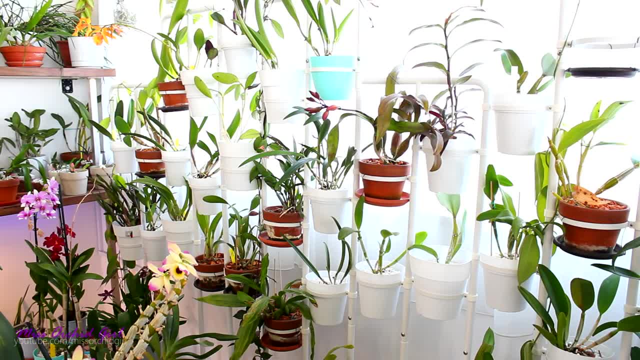 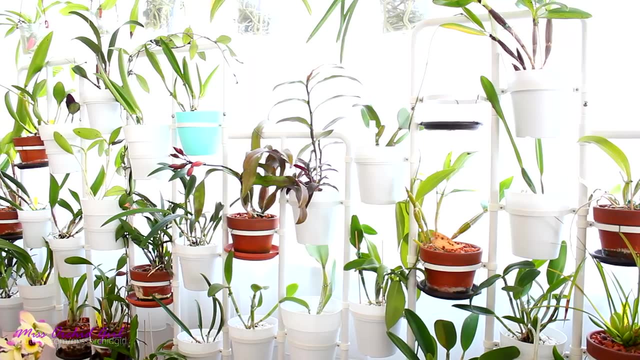 Vanda orchids. Also, many Catleas are not adapted to withstand hotter sunshine, So in this case, just to play it safe, it's always a good idea to provide filtered sunshine. So I have my high-light orchids really close to the window- and this is a southern window, but I do have a sheer curtain. 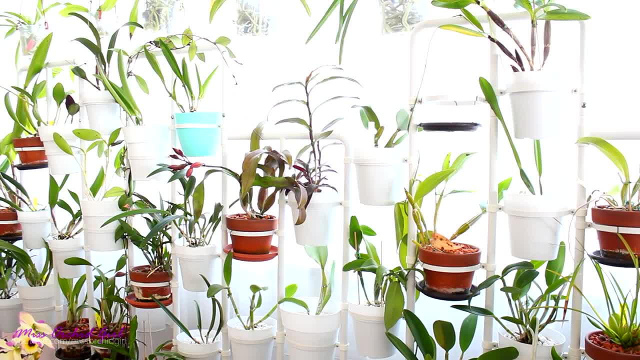 which protects me from direct sunlight. So I have my high-light orchids really close to the window, which protects them from overheating. But to wrap it up with high-light orchids, they will definitely not perform their best in low or even medium light conditions. Some of them might not bloom at all. 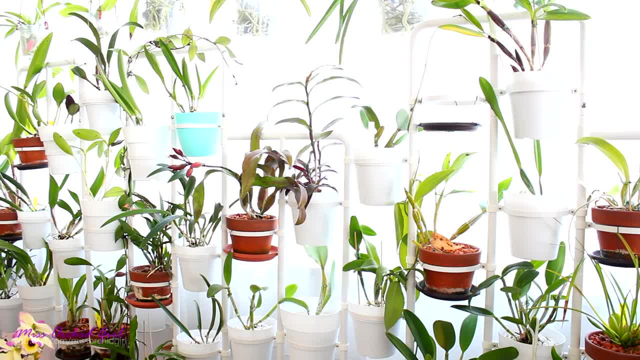 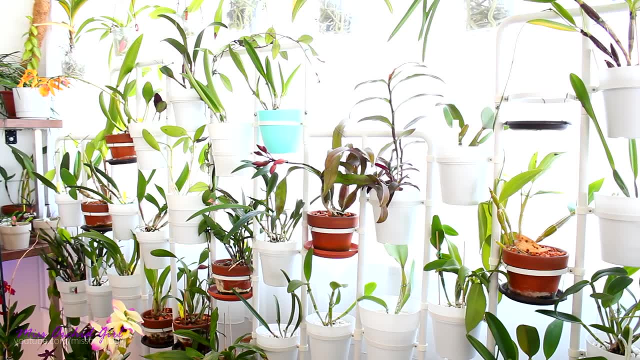 they might just grow foliage, while others might grow very, very slow. So these orchids are suited for those locations which benefit from a position that receives direct sunshine, And from there we can choose to filter that direct sunshine with a sheer curtain or even a shading cloth. but 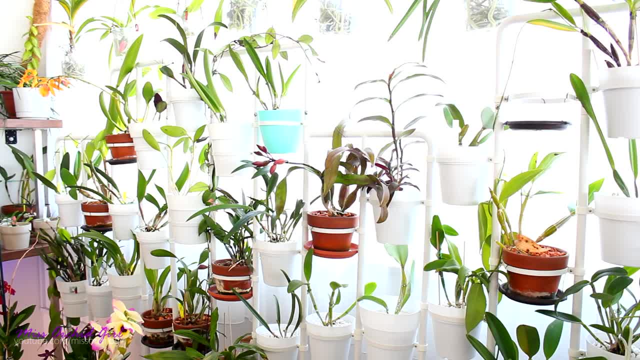 definitely never block the entire corner of the orchid. So if you have a high-light orchid you can try to filter it with a sheer curtain or even a shading cloth, but definitely never block the entire quantity of sun. The main problem with the quantity of light is sunburn, and sunburn usually. occurs when leaves of orchids overheat. Certain species of orchids cannot tolerate the same heat as other species. Usually, the high-light orchids are not as prone to sunburns because they can tolerate their leaves heating up, at least to a certain extent, while let's say, low-light 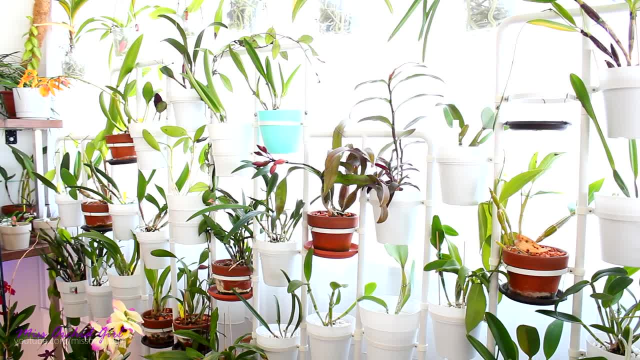 orchids cannot tolerate the same amount of heat as a high-light orchid. I do actually have a video which explains a little bit more how plants, and, of course, orchids, protect themselves from overheating of the leaves. Overheating damage is irreversible. Once it happened, it can never go. 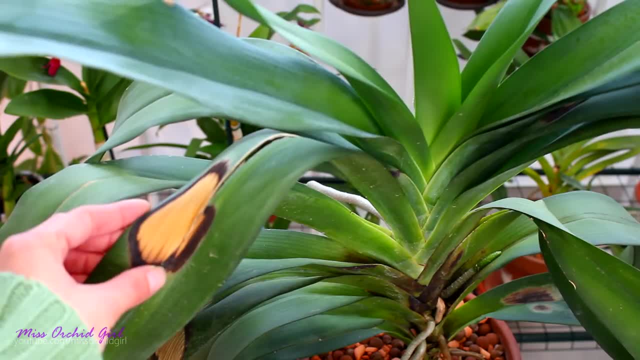 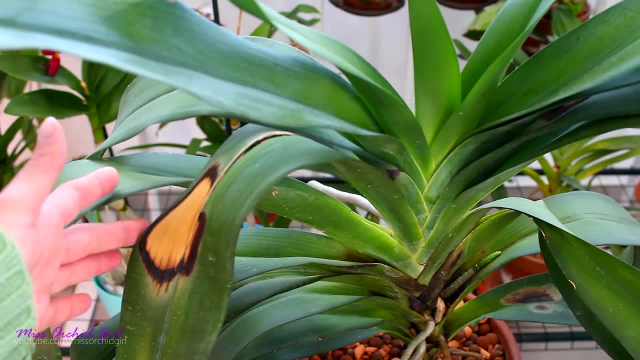 back. The leaf can never repair itself, And not only does it look pretty bad, but it also affects the health of the orchid. Leaves are responsible with photosynthesis. If a certain part of the leaf is completely destroyed, it will definitely not perform photosynthesis. So here I have a pretty 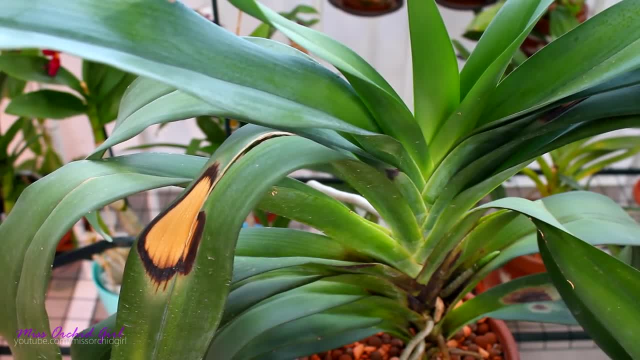 common problem. Now this happened because it received direct sunshine when the temperature around it was really hot. Colder air and winds can decrease the temperature on the leaf surface and can also minimize the effects of direct sunshine. So let's take a theoretical example. We have a 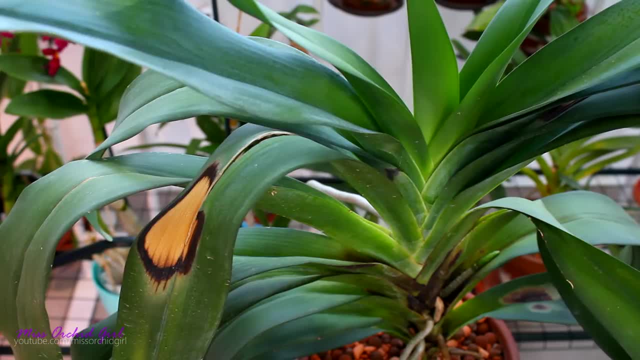 high-light orchid, which receives direct sunshine, but the ambiental temperature is around 15 degrees Celsius or 20 degrees Celsius. It also has ventilation. Well, that orchid is far less prone to get sunburns than the other orchids, which is why it is called a high-light orchid. But the higher the temperature is around the orchid, the more prone the orchid will be to get sunburned. In higher temperatures the leaves cannot cool off as much as in lower temperatures, So the quantity of direct sunshine can affect orchids depending solely on their environment- Another thing to keep in mind. even with high-light orchids, is that if they are grown in an environment which receives quite the clear distinction between summertime and wintertime when it comes to quantities of light, after the winter they will not be prepared to handle direct sunshine as well, let's say, as in the summertime. They need to be gradually adjusted to the spring sun, And this is because they need some time to develop and release the certain chemical that protects their leaves from being burned, And if you watched the video that I mentioned earlier, you can find it in the description below, If you're. 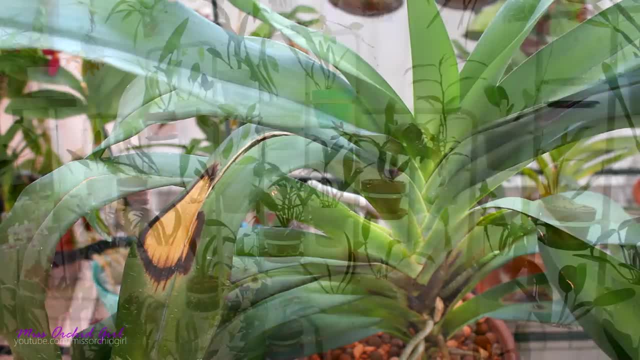 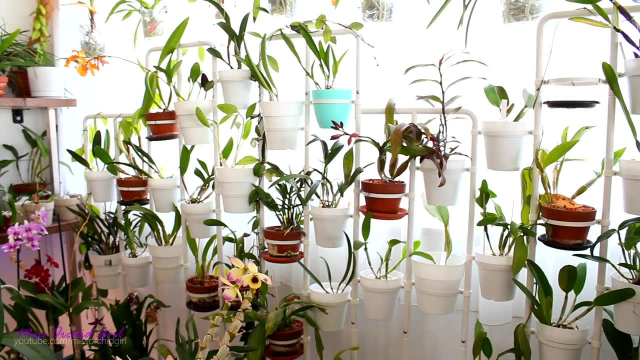 going to find it in the description. you'll see exactly what I'm talking about. The higher the amount of direct sunlight, the more the leaves will heat up. So we need to consider the elements in our growing environment, such as humidity, ventilation and temperature, so we know if our orchid, even if 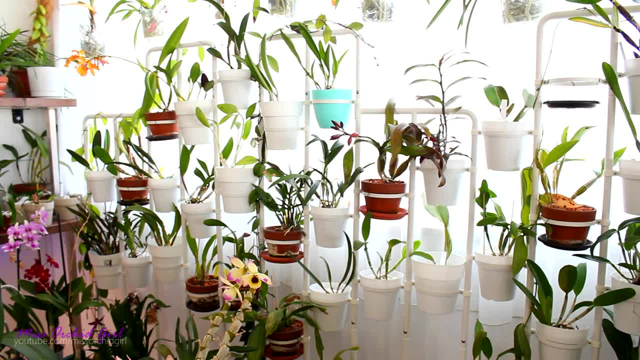 it's a high-light orchid is prone to getting sunburned. Light is an element all plants need to perform photosynthesis and have energy to grow, So priving orchids from light, even low-light orchids, is never a good idea. And that's about it on this video. If you liked this video, feel free to rate, comment and subscribe to my channel And I'll see you in the next one. Bye. 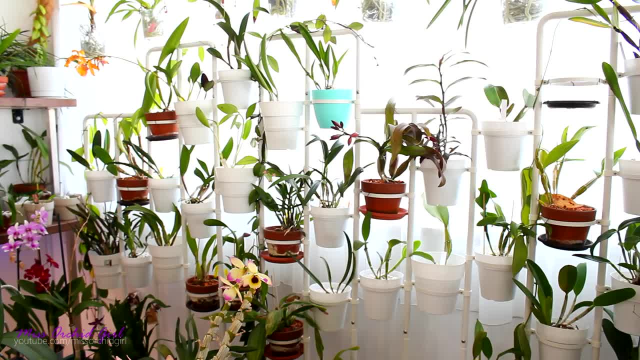 on the light quantity. I tried to keep this as simple as possible, but I will finish by saying that there are certain instruments that measure the quantity of light you have in a certain location. I'll link you down below to such a product and also in the description I will. 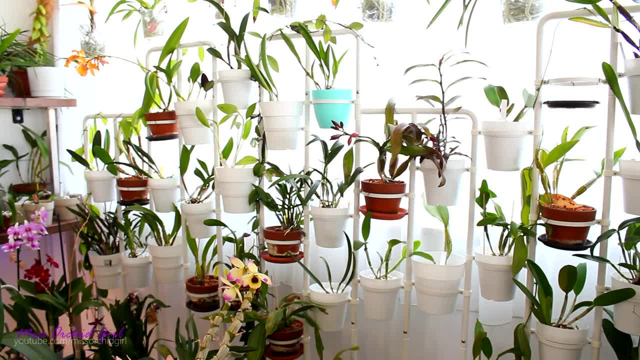 classify the low light orchids and the highlight orchids and tell you their requirements in foot candles, which is the unit of measure that the device uses. so if you have that device or would like to buy one, at least you'll have a reference point. I have such a device, but 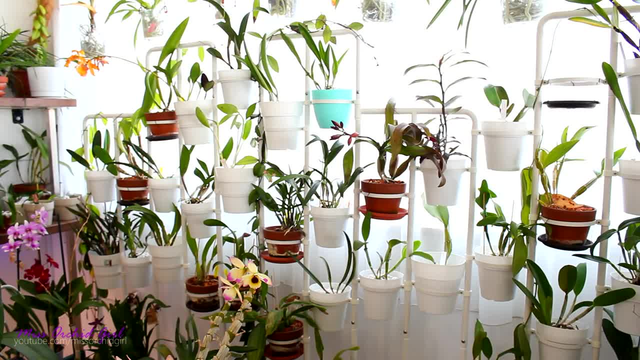 I've never used it. I am more of an intuitive person- but definitely those devices are really helpful. so check the description down below if you're interested. so thank you so much for watching this video. hope you've enjoyed it and thank you for suggesting it if you liked the video, please. 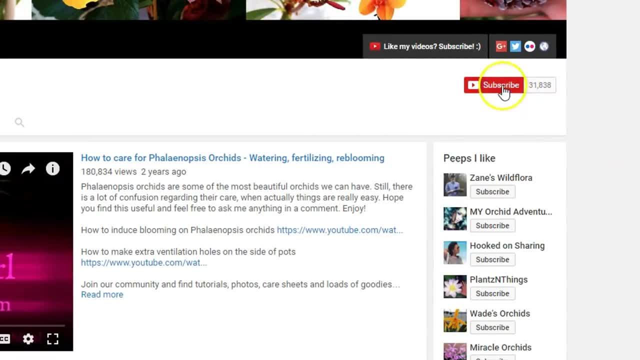 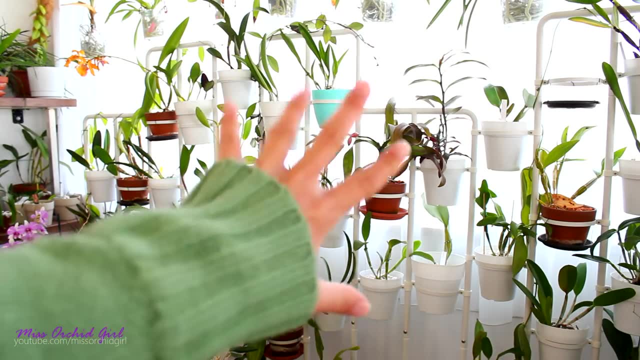 give it a thumbs up if you didn't give it a thumbs down. subscribe to my channel for more orchids and plants videos and don't forget to turn on notifications so you never miss a video. and with that said, I'll see you all next time. bye, now. if you remember one of our older discussions, 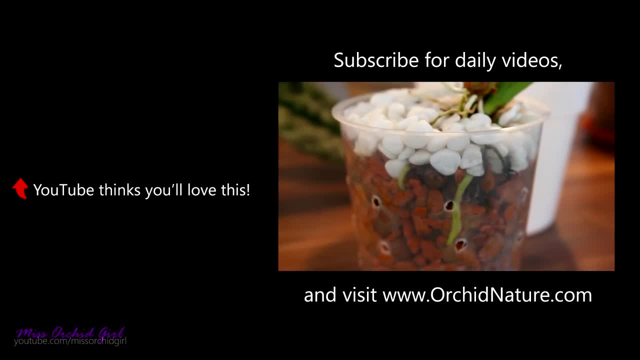 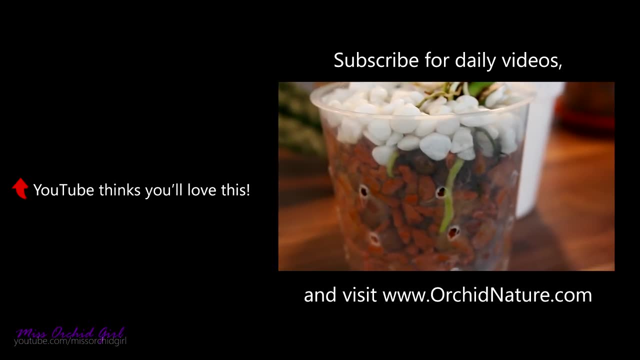 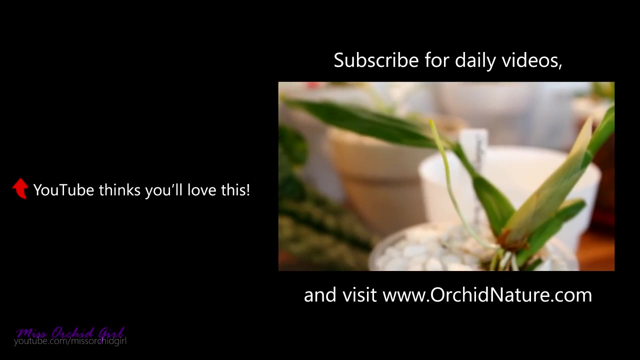 regarding how roots grow, I told you that the pattern is pretty random because, except for obtaining moisture and nutrients, roots need to anchor orchids as well. well, here's a funny example of that. here we have the selagineus sitana, with a few roots going inside the medium and one just reaching for the sky. this is very normal with. 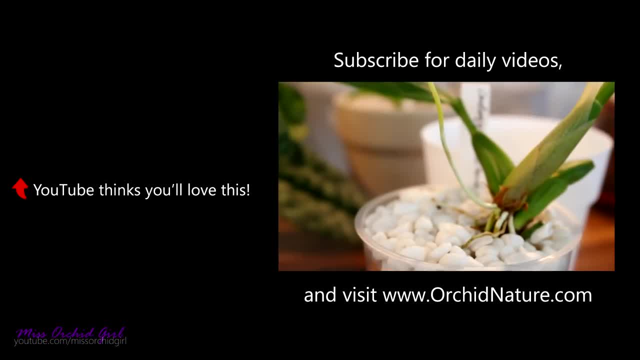 epiphytic orchids. so if you have an orchid which displays these symptoms, don't worry, it's perfectly normal. roots will pretty much tend to do whatever they feel like doing. 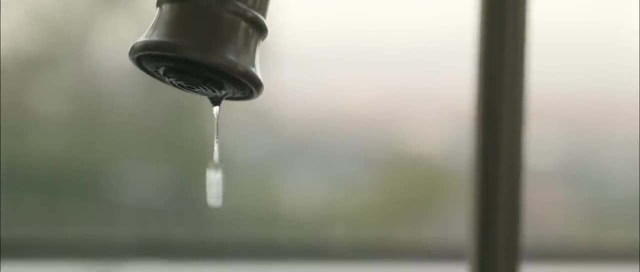 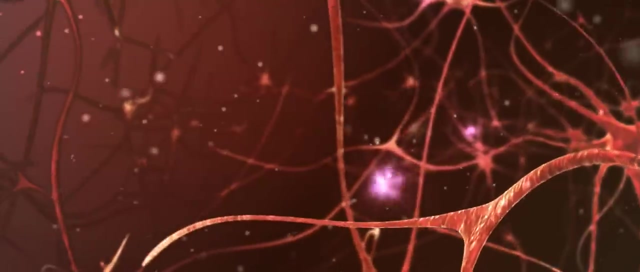 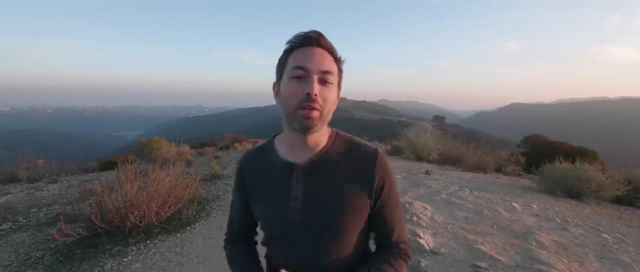 What's the connection between a dripping faucet, the Mandelbrot set a population of rabbits, thermal convection in a fluid and the firing of neurons in your brain? It's this one simple equation. This video is sponsored by Fast Hosts, who are offering UK viewers the chance to win a. 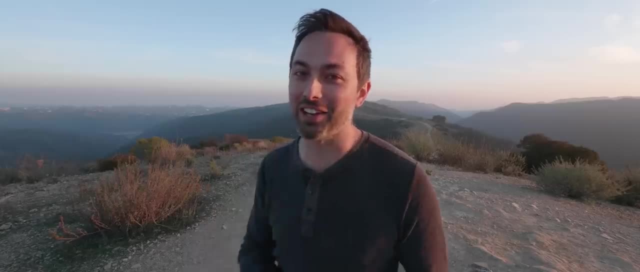 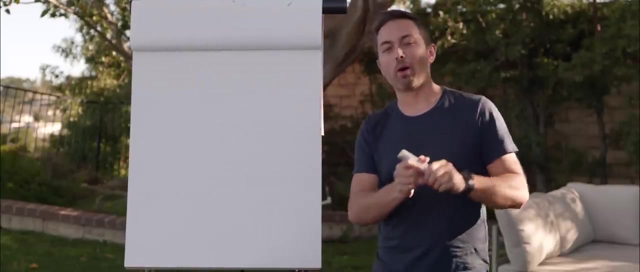 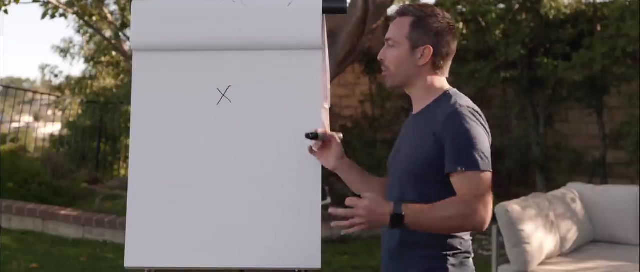 trip to South by Southwest, if they can answer my question at the end of this video. so stay tuned for that. Let's say you want to model a population of rabbits. If you have X rabbits this year, how many rabbits will you have next year? Well, the simplest model I can imagine is where we just 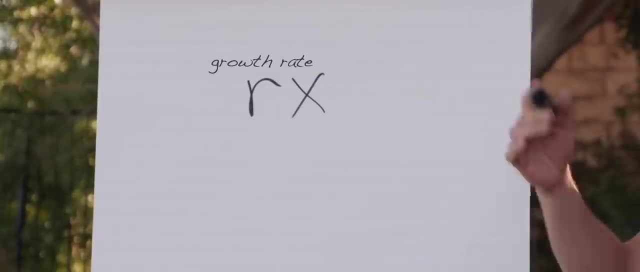 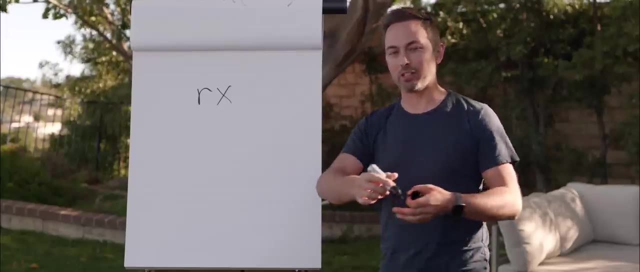 multiply by some number, the growth rate R, which could be say 2,, and this would mean the population would double every year, And the problem with that is it means the number of rabbits would grow exponentially forever. So I can add the term 1 minus X to rabbit.